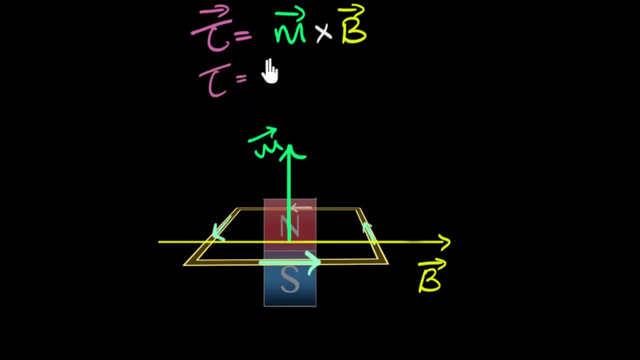 So the magnitude says, if you look at the magnitude, the magnitude of tau would be equal to magnitude of m times b times for a cross product. there's a sine, So there'll be times sine of the angle between m and b. 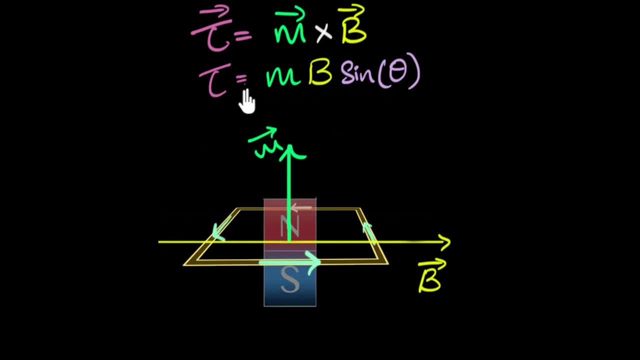 So if we call that angle theta, it'll be sine of the angle between them. So this is saying that if you have more magnetic moment, you'll get more torque. Does that make sense? Well, yeah, If you have stronger current. 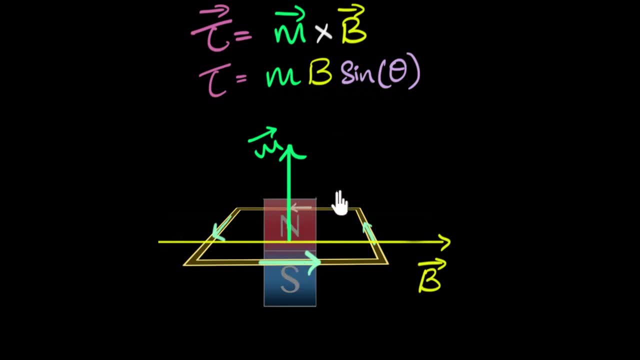 if it behaves like a stronger magnet, you will expect more torque acting on it. On the other hand, if it behaves like a weaker magnet, less torque. If there is no magnet at all, obviously it will not be affected by the magnetic field. 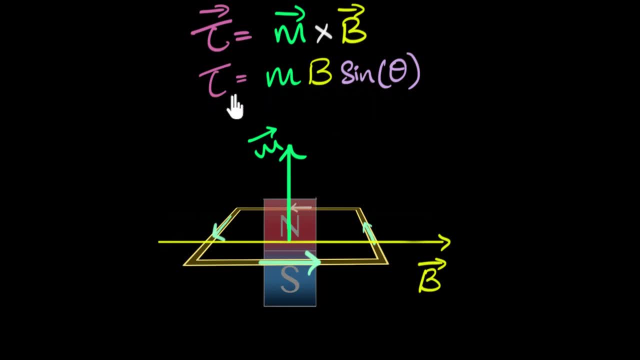 so torque would be zero. So that makes sense. The equation is also saying that the torque would increase with the strength of the external field that we apply. That also makes sense, right? If you apply a very weak field, there'll be a very weak turning force. 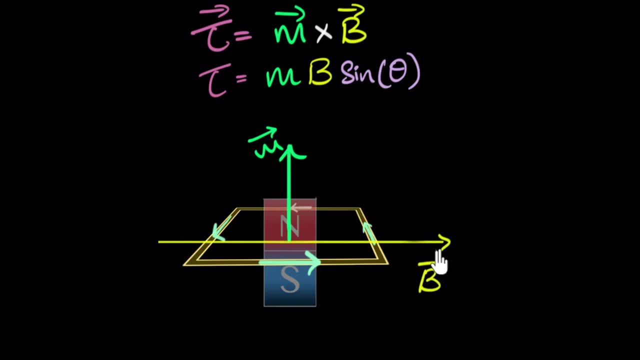 Strong field would provide a strong turning force, And if you don't provide any field at all, it'll not turn at all. So that also makes sense that the torque depends upon the magnetic field. Finally, it says that the torque also depends on the magnetic field. 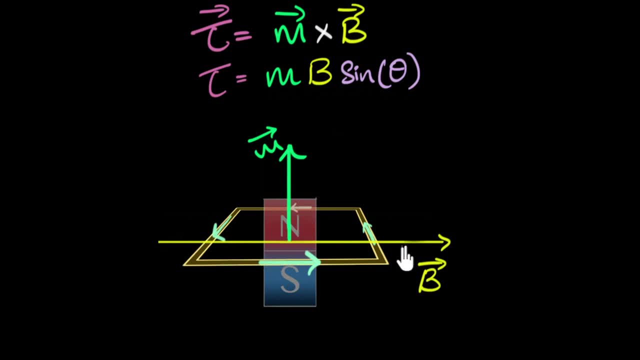 It depends upon the sign of the angle between the two. What does that mean? Well, let's look at it. In this particular case, theta, the angle between m vector and b vector is 90 degrees. So the equation is saying that the torque is maximum. 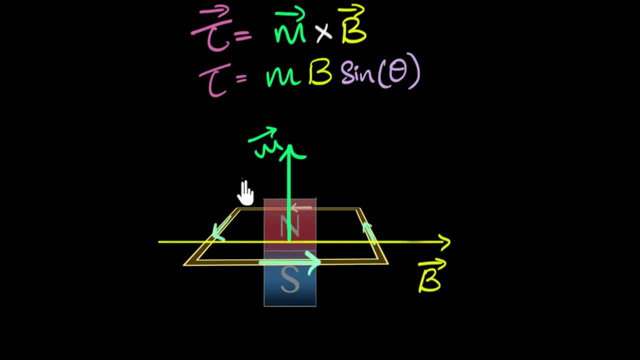 And now it says that in this position, because of the torque, our coil is going to turn, And because it says m cross b, it is saying that m is going to turn towards b, So the torque will act this way And notice as the coil turns. 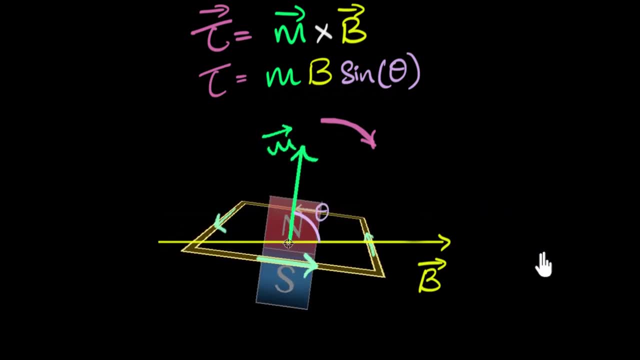 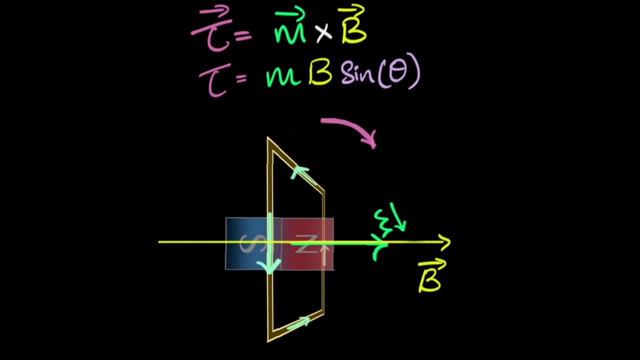 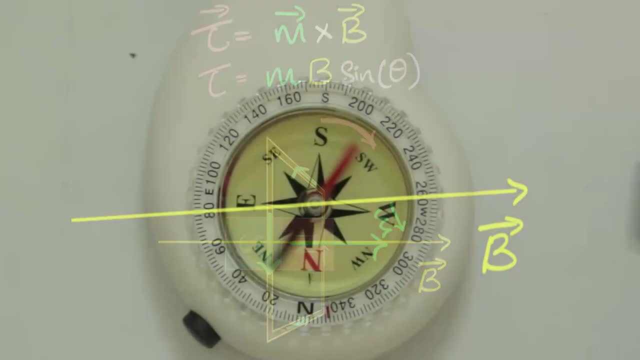 theta becomes zero, the torque would be zero. So once in this position, there'll be no longer a torque acting on it, And if you think about it, that kind of makes sense. That's exactly what we saw in the intro. We saw that when the needle was not aligned. 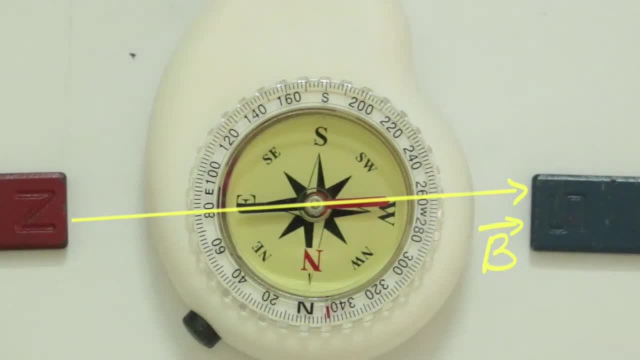 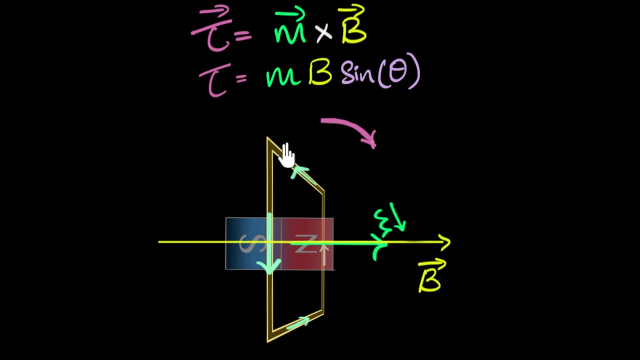 with the magnetic field there was a torque, But once the needle gets aligned, it stays there, meaning the torque becomes zero. So you see what the field is trying to do. The field's job is to align the magnetic moment, or to align the magnet in the direction of the field. 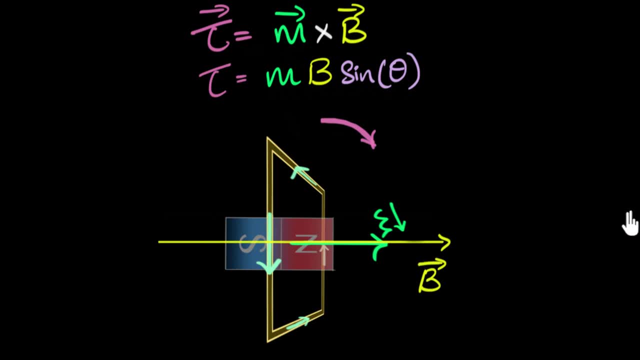 That's why, when it's completely aligned, the torque becomes zero, And when it is at perpendicular, when it is perpendicular, that's when the torque becomes maximum, because it is the exact opposite of being aligned: perpendicular. So the field hits it and puts a maximum torque. 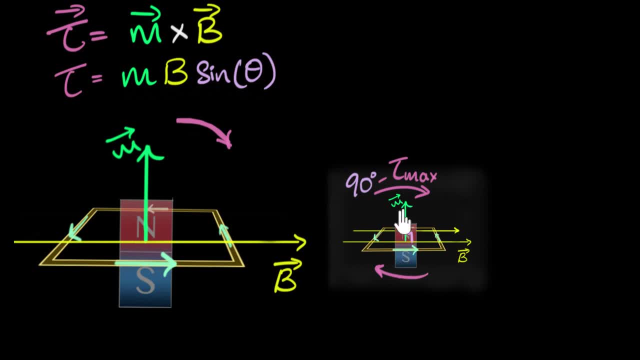 So here's what we saw: When we have 90 degrees between M and B, the torque is maximum, And when the M is aligned with B- zero degrees- the torque also becomes zero. Now be careful over here. You might think: hey, wait a second. 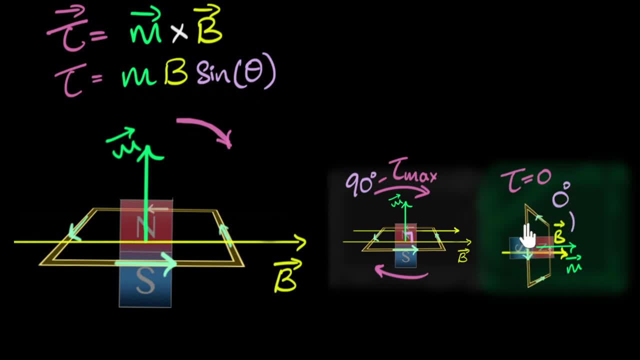 In this case, why are we saying it's zero degrees? The plane of the coil is perpendicular to the magnetic field, right? Well, yeah, but remember, the angle is not between the plane and the field. The angle is between the M vector and the field vector. 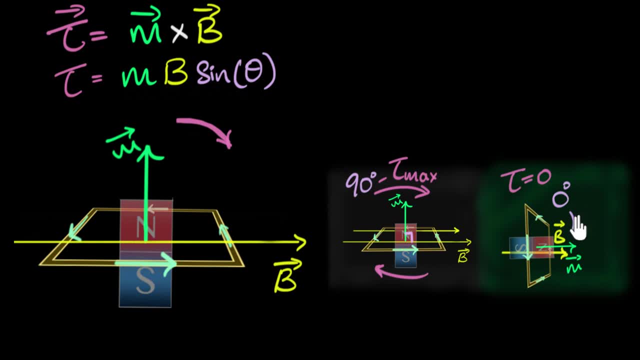 Got it. So that's where I used to always get confused, especially in numericals. So remember, this is the angle between the M vector and the B vector, not the plane and the B vector. And to give you some intuition behind this, 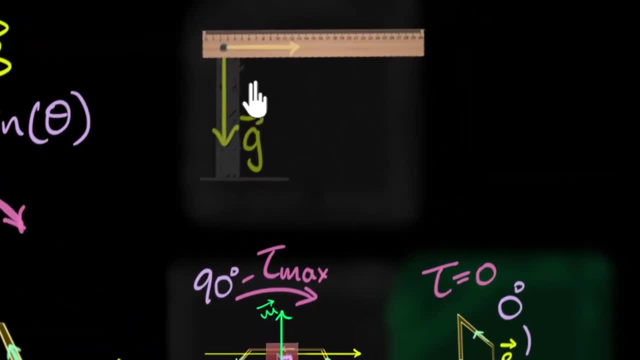 let me give you a familiar example. Consider a pendulum. Basically, you know, imagine you have a pendulum. Imagine you have a ruler. you made a hole in that and you hung it somewhere. Now, in this position you can kind of see that gravity is going to put a torque. 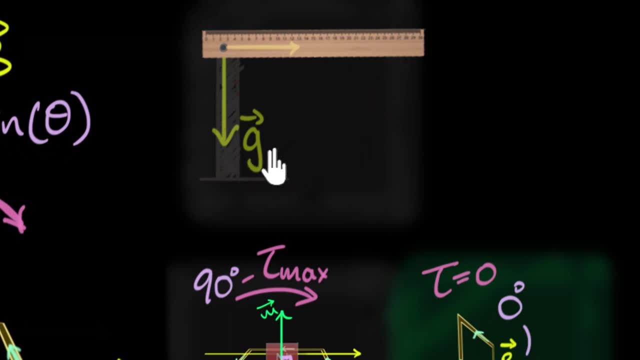 on it in this direction and tries to turn it over here. But as this ruler turns, let's turn this ruler. As this ruler turns, you know in your bone that now the torque starts decreasing, decreasing, decreasing And eventually, when it's aligned, in this position. 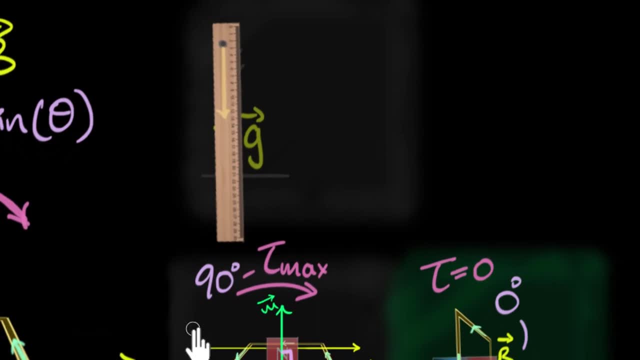 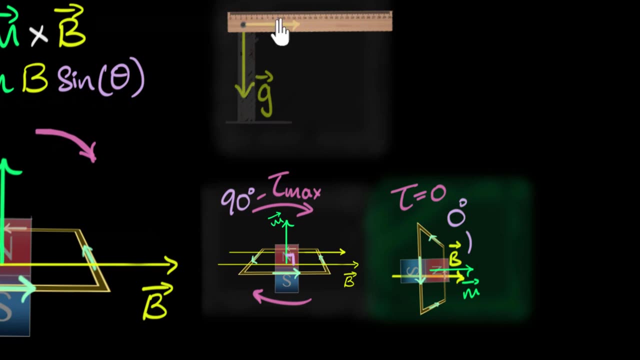 that's when the torque is zero. Exactly same thing happening over here as well. Exactly same thing happening over here as well. Exactly same thing happening over here as well. Gravity wants to align the ruler in its direction, And that's why, in this case, 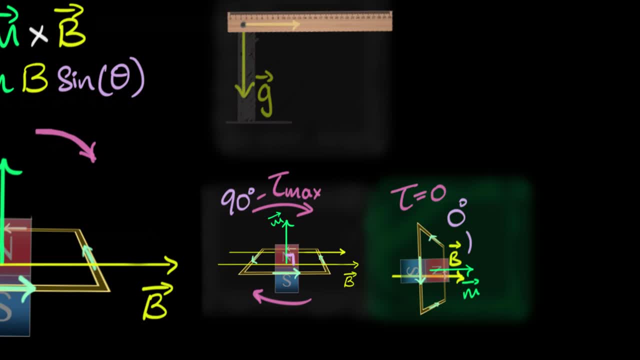 we have the maximum torque 90 degrees, And when it's aligned we get zero torque. The field is trying to align the ruler. Here. the field is trying to align the M vector. That's why it's putting the torque. 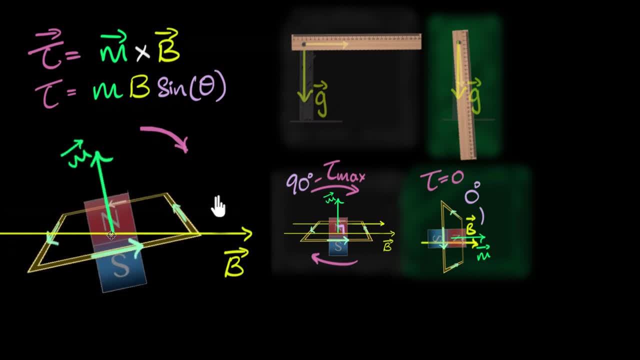 Okay, what if the angle is more than 90 degrees? In this position, what do you think happens to the torque? Would it be more? Would it be more Than when it was perpendicular or less? And can you imagine what will happen? 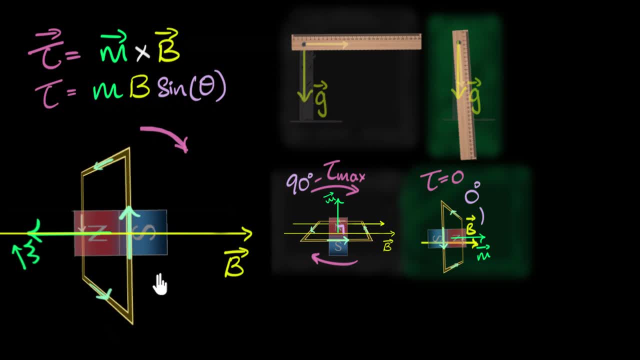 if we were to turn it this way and keep it in this direction, Go ahead. Why don't you pause the video and think a little bit about what happens in those cases? All right, if you're given this a shot, let's see. 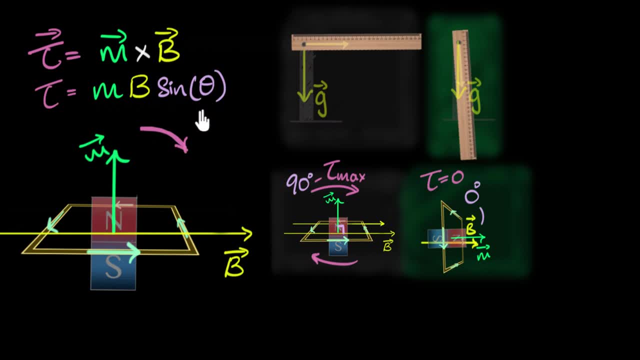 If the angle becomes more than 90 degrees, again sine value will start reducing Because sine has the maximum value at 90.. Sine 90 is one right. So above 90 degrees, again the torque starts reducing, reducing, reducing, reducing. 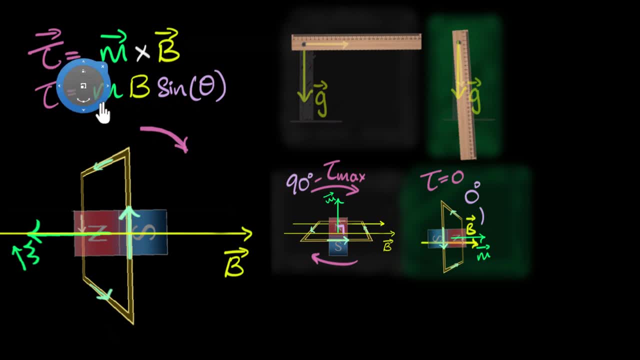 And in this position the angle between B and M is 180 degrees and sine 180 is also zero. So even in this position the torque is zero. So even at 180 degrees the torque becomes zero. But can you feel the difference between these two cases? 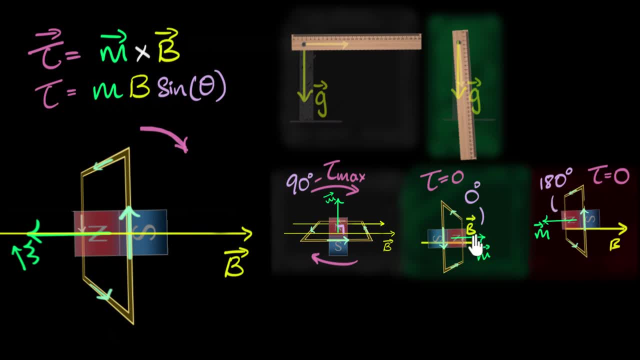 In both these cases torque is zero. but there's some conceptual, fundamental difference between these two positions. Again, I want you to pause the video and think a little bit about this. Maybe you can use the ruler example and see if you can figure out what difference you find. 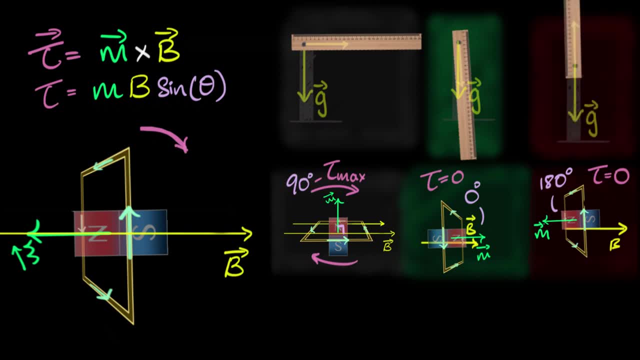 All right. if you think in terms of the ruler, this is exactly like trying to put a ruler and balancing it this way. Even in this situation, the torque on the ruler would be zero. If you can exactly balance it, it would be zero. 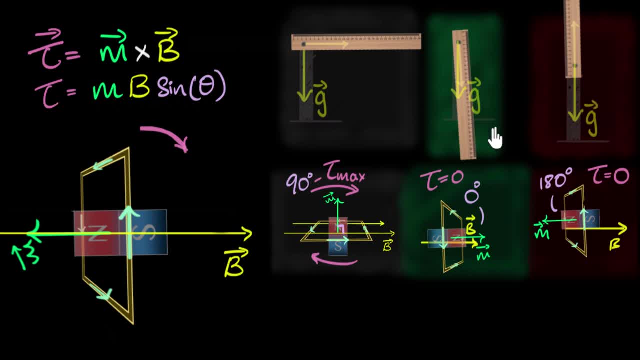 But you can feel in your bones the difference between these two. right, This is a very stable position. What I mean is, if you were to nudge it a little bit, the torque acting on this will bring it back to this position. 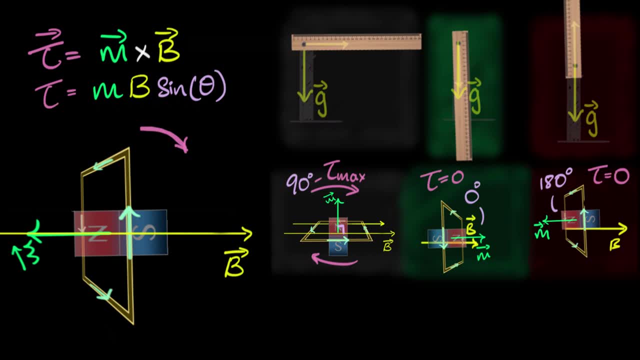 This is a very stable equilibrium position. we would like to say, On the other hand, if you disturb this equilibrium, even a little bit, the torque will not bring it back. The torque now that equilibrium position is lost and the torque will turn it all the way. 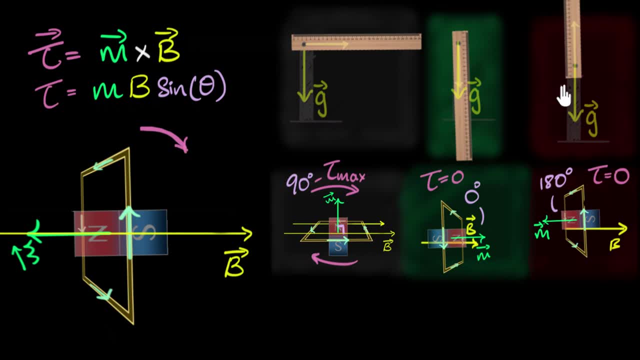 to the stable position, And that's why, even though this is an equilibrium, we call this as unstable equilibrium. You disturb it a little bit and it's gone, And that's why this gives you that unsettling feeling. right, Because this is a very delicate balance. 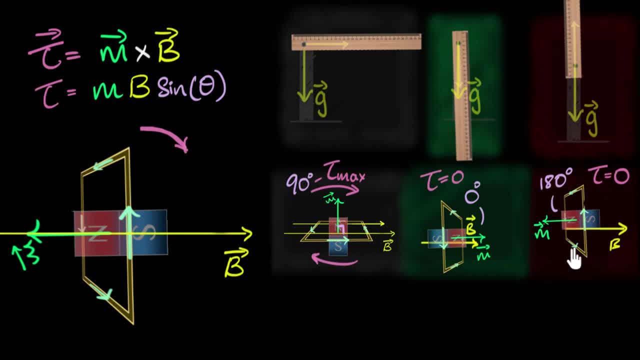 You disturb it and it's gone. Something very similar is gonna happen over here as well. This is an unstable equilibrium position, Meaning if we were to disturb this even a little bit, then the torque will put it in this position, the stable position. 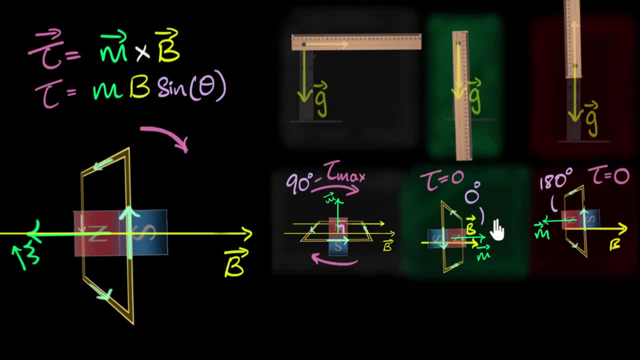 So the big difference is, even though the torque is zero in both these cases, and they are in equilibrium, this is an unstable equilibrium and this is a stable equilibrium. And finally, I want you to think about energies associated with these two equilibrium positions. 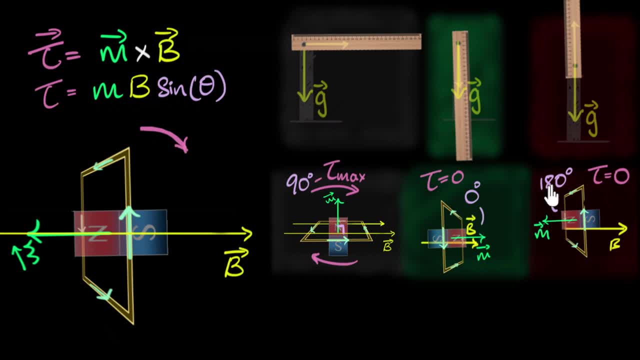 Can you pause the video again one last time and think about which of these two positions would have higher potential energies? And again the ruler might help you. So pause the video and think about which of them has a higher potential energy. 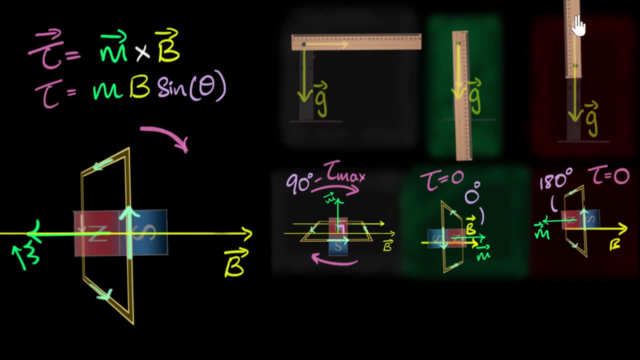 All right, you might know already that, when it comes to gravity, more height means more potential energy. Since the ruler over here is higher than over here, there must be more potential energy over here, and there must be less potential energy over here. 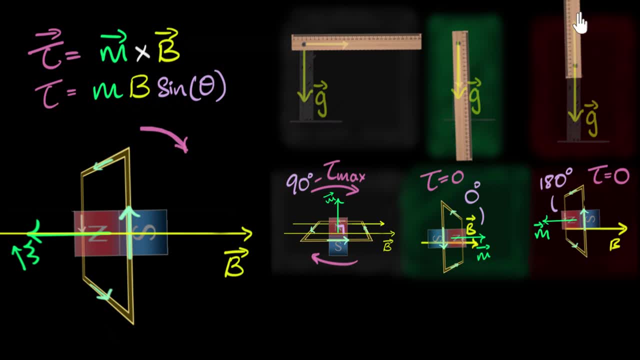 So you see, in the unstable equilibrium state, the objects tend to have higher potential energy. And what is nature trying to do? Nature is trying to put a torque and reduce the potential energy and get it to stability. It's that potential energy which gets converted. 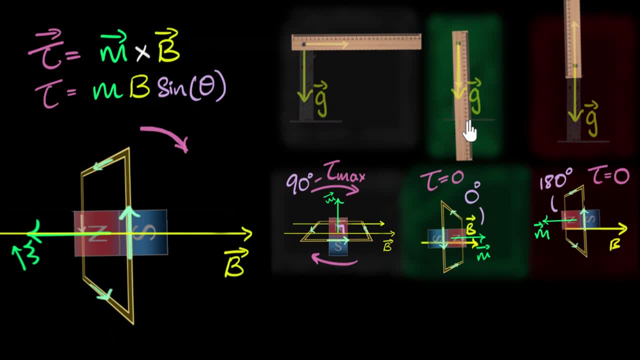 to kinetic energy of rotation, at least in this case, and maybe eventually it'll get dissipated as heat, And the same thing applies here as well. When the magnetic moment is in the opposite direction of the field vector, we are at the maximum energy. 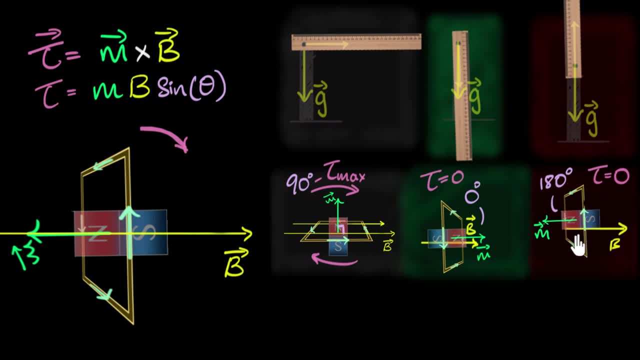 This has a very high potential energy and nature hates that. And so when you disturb this equilibrium position, then nature puts a torque on it and goes from high energy- sorry, unstable equilibrium state- to the lowest energy, stable equilibrium state. And with this knowledge of torque,